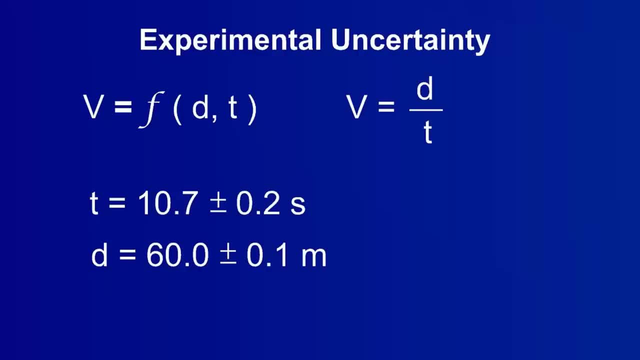 but rather from physical equipment limitations, such as the spacing of teeth on a gear inside of the device. Uncertainty can be given within a word problem or, more commonly, as a value that is added to or subtracted from the measurement, as shown. 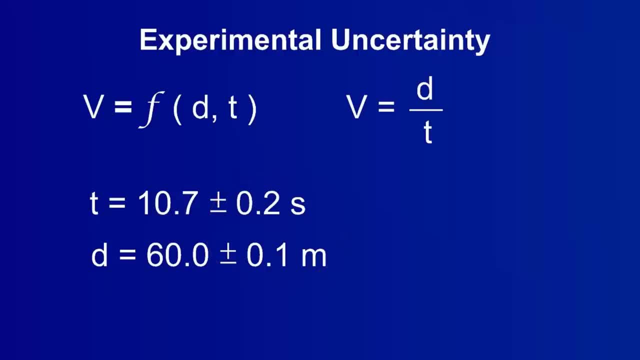 All experimental measurements have uncertainty, though it is not always shown. The velocity calculated from these measurements will also have an amount of uncertainty. The uncertainty of a resultant is a function of the uncertainties of all the measurements used to calculate it. Uncertainty is represented with the level of uncertainty. 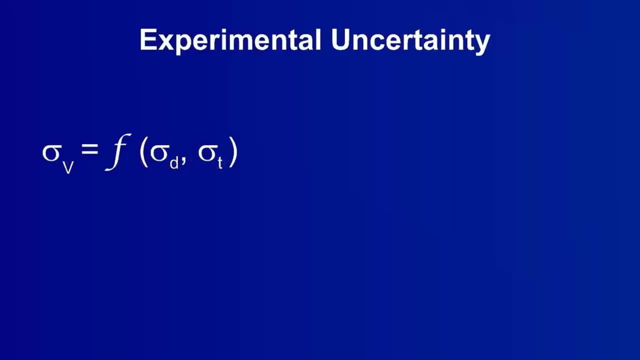 Uncertainty is represented with the lowercase Greek letter sigma. Let's look at the uncertainty of the velocity. It is equal to the root sum of the squares, or RSS, of a contribution from the uncertainty of the distance and a contribution from the uncertainty of the time. 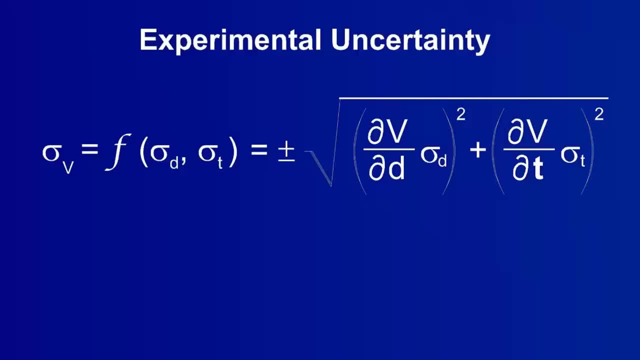 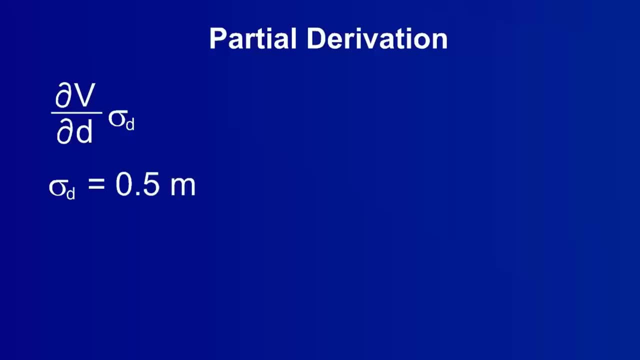 Let's take a closer look at one of these contributions. Sigma sub d is the uncertainty of our distance measurement. This other term indicates to take the partial derivative of the velocity v with respect to the distance d Recall the equation for the velocity. 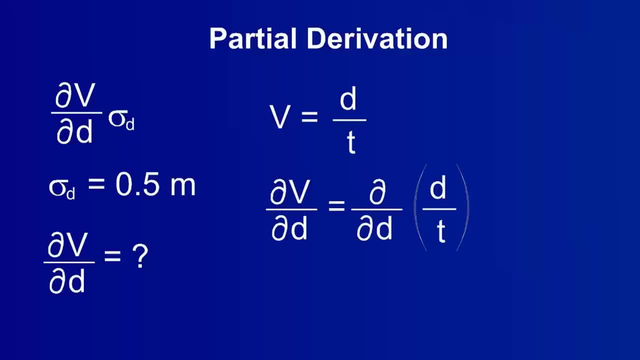 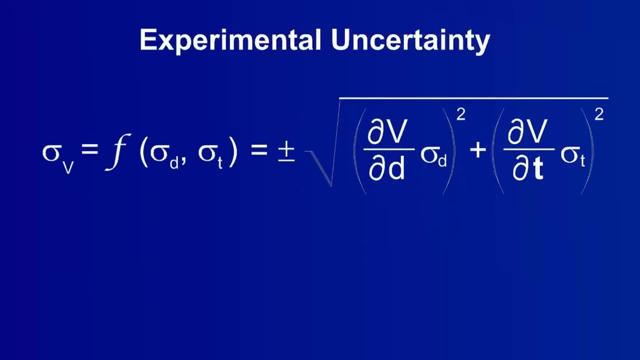 To take the partial derivative, treat all variables other than the variable of interest d as if they were constants and take the derivative with d as the variable. The partial derivative with respect to the time t is also needed Because the time is in the denominator. 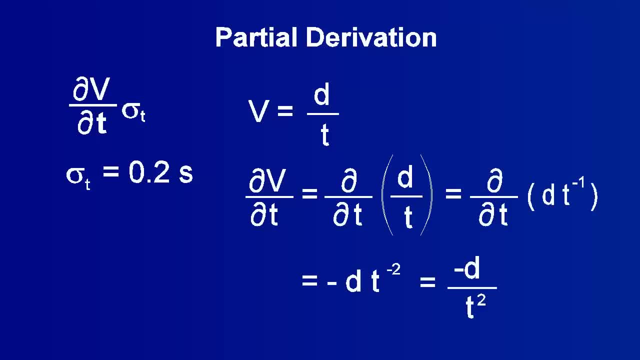 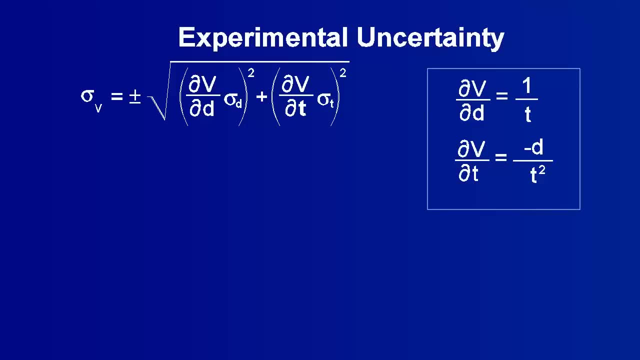 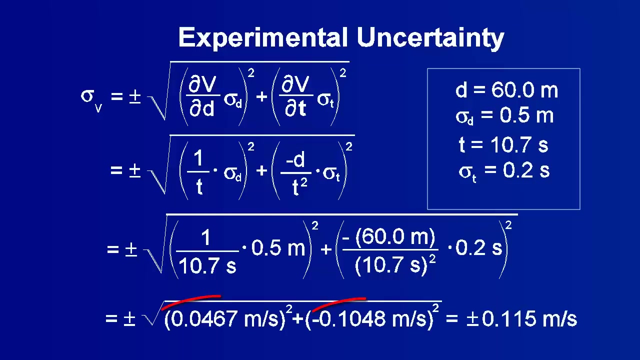 its partial derivative is a bit more complex. Now the uncertainty of the velocity can be calculated. Recall the partial derivatives and substitute them in. Recall the time distance and their uncertainties. Substitute these values in as well, Based on the two contributing factors seen here in the root sum of the squares. 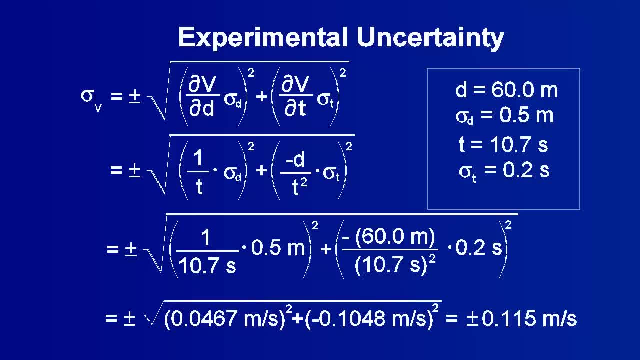 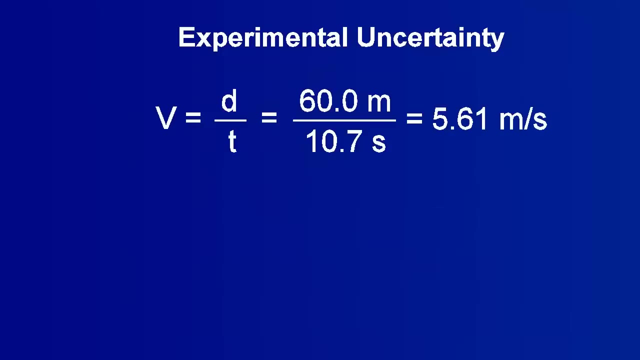 which of the two measurements has a larger effect on the uncertainty of the velocity? If more accuracy is needed for the velocity, which measurement needs to be more accurate? Note that the uncertainty of the velocity can be calculated independently of the velocity itself. Calculate the velocity and report the solution in the proper format. 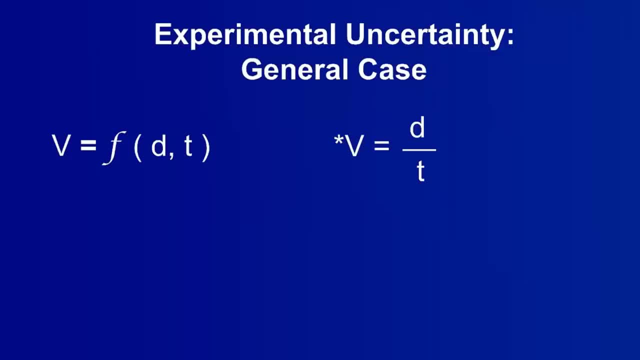 Many of these uncertainty calculation equations have been shown specifically for this example. Let's expand these equations to include any general case. The resultant r is a function of variables x sub 1 through x sub n. This may be any function with any variables. 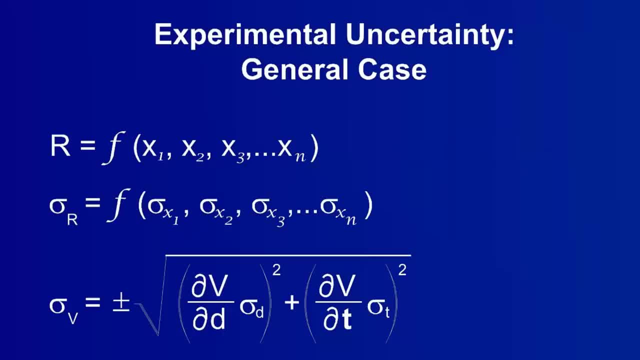 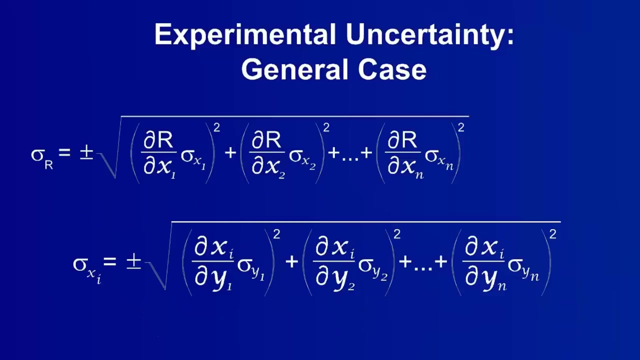 The uncertainty of r is a function of the uncertainties of all of those variables. This function is always. the uncertainty of r is equal to the root sum of the squares of the partial derivative of each variable multiplied by the variable's uncertainty. If one of the variables used to calculate 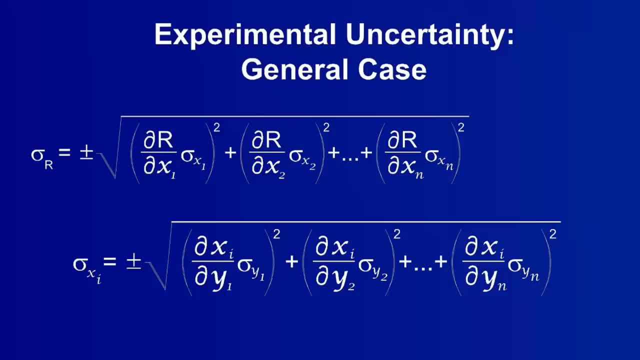 the resultant is itself calculated from another measurement or measurements y sub i. then a local uncertainty analysis must be done on that variable, x sub i, which can be any of the variables x sub 1 through x sub n, to find its uncertainty before solving for r. 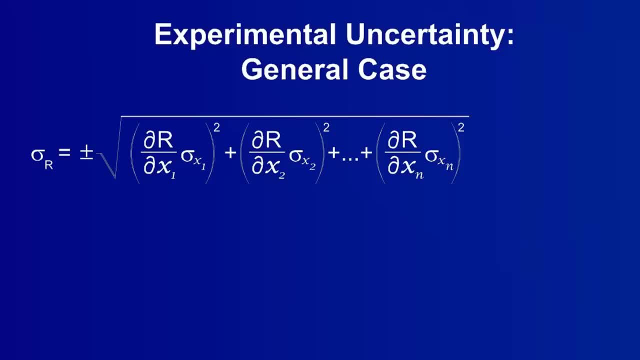 Lastly, there is another way to report uncertainty. Relative uncertainty, or U is a percentage. It is equal to the uncertainty of r divided by r. This indicates the accuracy of the observation or experimental measurements scaled to the resultant. For example, an uncertainty of 0.5 meters. 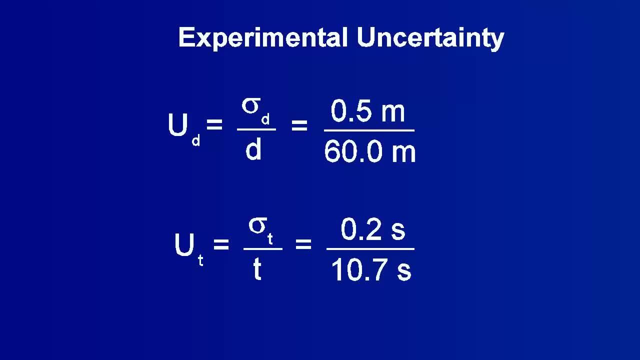 over a distance of 60 meters indicates far more accuracy than an uncertainty of 0.2 seconds over a time of 10.7 seconds. Let's rearrange the equation for the velocity uncertainty: The partial derivative of v with respect to d.